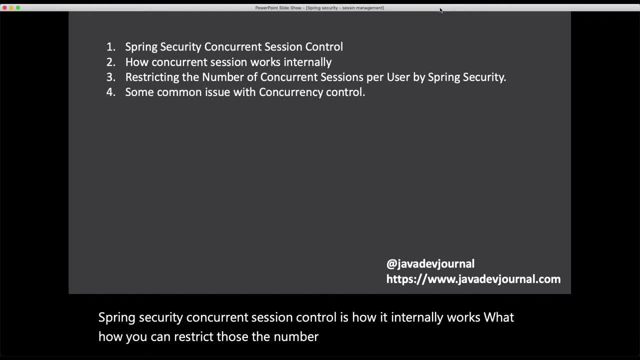 you can restrict those- a number of concurrent sessions, and then some of the common issues, or not the issues, but in the sense that what are the different things? are the precautions, are the points which you should be clear on right. So we will see some of the configuration- default configurations, customization point- and then we will get into a deeper details, dig into the internal working of the spring security. In order to do that, we will again go back to 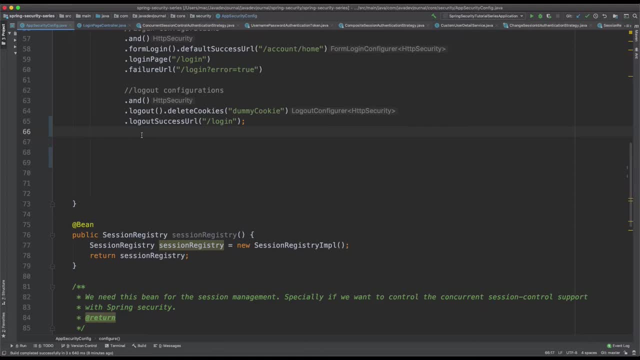 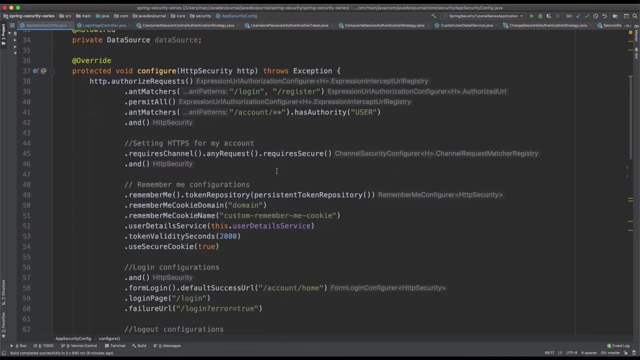 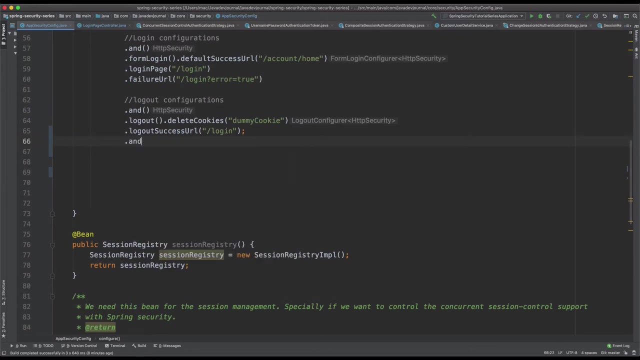 our main spring security configuration file. So our file, as usual, is extending. the web security configuration adapter and all the related spring security control will go into this class, right, And we will continue extending our session control thing. Okay, Let's move this one, Okay, And then we will continue to using our session management thing. So this session management aspect controls like your session management. 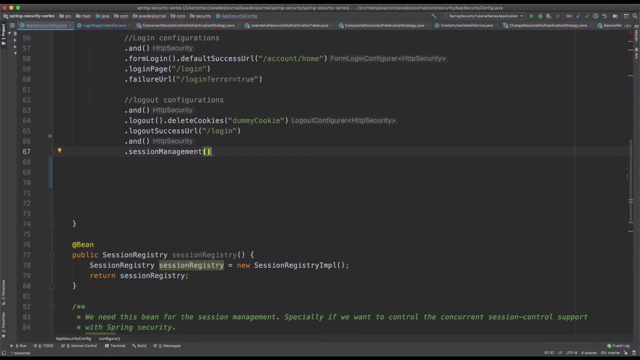 validations, then this concurrent session control and then in next chapter, we are going to talk about the uh, the spring, uh, security, session management or the session fixation things, right, okay. so, in order to control the maximum session, this is the property maximum session and in this one, uh, you, it's taken, takes an integer and you can tell spring that what is the maximum. 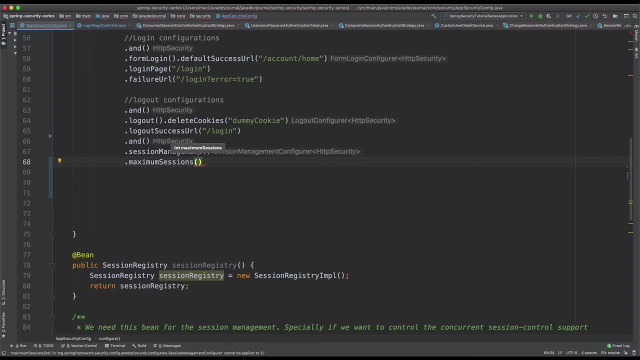 session you want to allow per customer. it's not about entire application, it's about per customer or the locked in customer right by default, uh, there is no restriction. so if you don't specify this thing, uh, by default, spring security don't put any restrictions. so you can do, you can log. 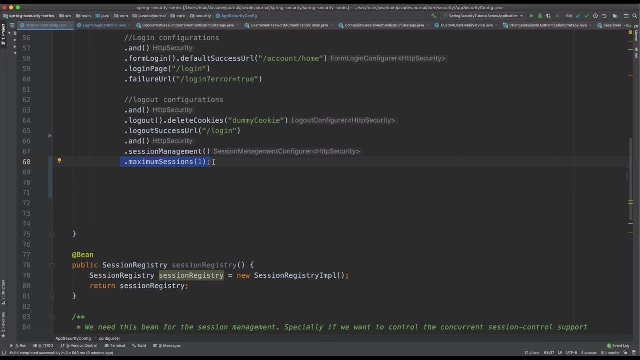 in from n different places and spring security won't control. uh, won't complain about it, right? so now we have set the maximum session as one. so what we're going to do is: uh, this is the basic configuration for now. we will start our application and then see. 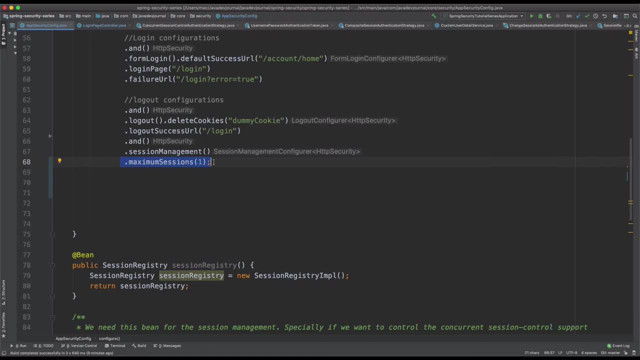 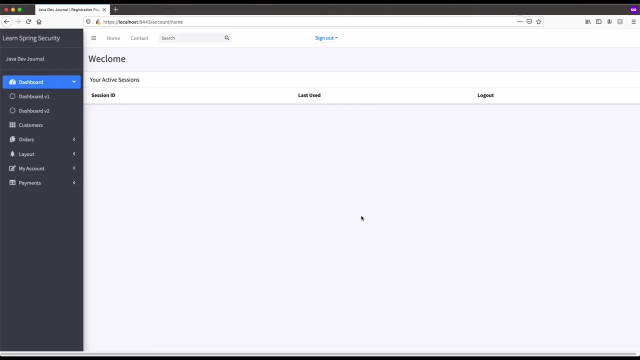 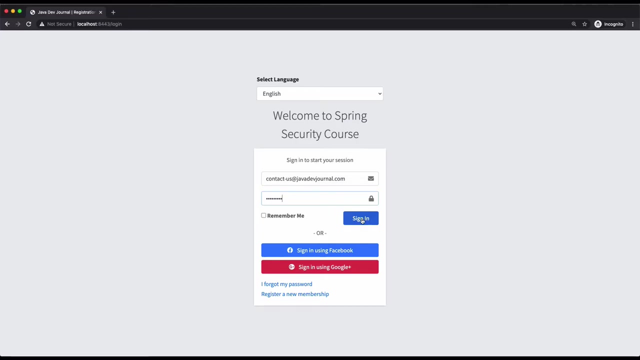 the behavior in action. what does what? what will happen if we set the maximum session to one, two, three, whatever? uh, you want to set right? all right, so i'm already logged from. logged in from the firefox. okay, let's try to do a login from a different browser. okay, so i'm on to the chrome. 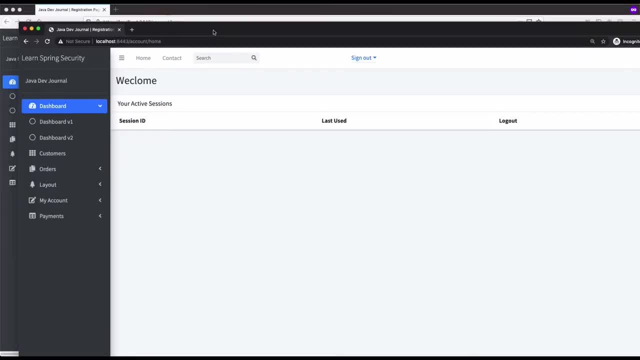 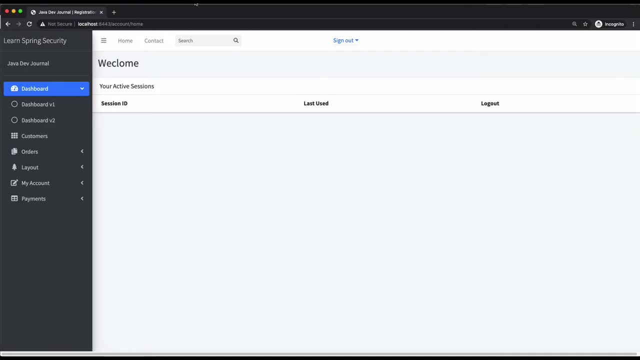 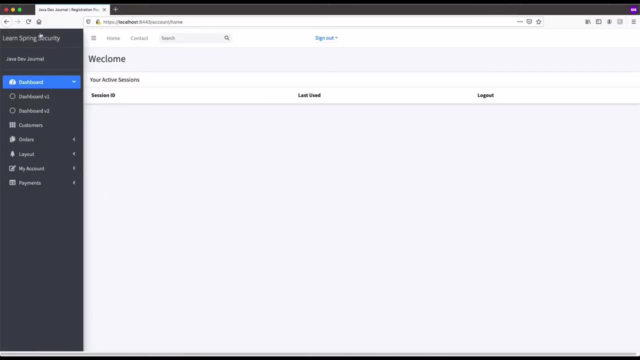 we'll try to do login. it works right. so right now i am technically logged in from two different places, one from the chrome and one from the firefox. okay, so let's try to do some action onto the firefox. okay, if i refresh it, everything works fine. now let's go back to firefox and do the same thing. 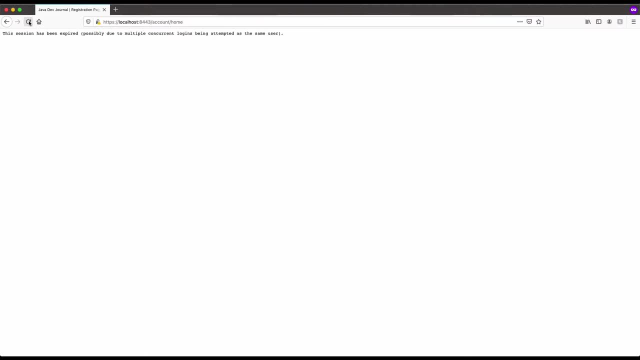 if i do a refresh, that means i am trying to take another action, assuming that i am already logged in, right. in this case, i will get this message, and this is the out of the box message right- which say, which tells the customer that, hey, you have already exceeded your limit, correct? so 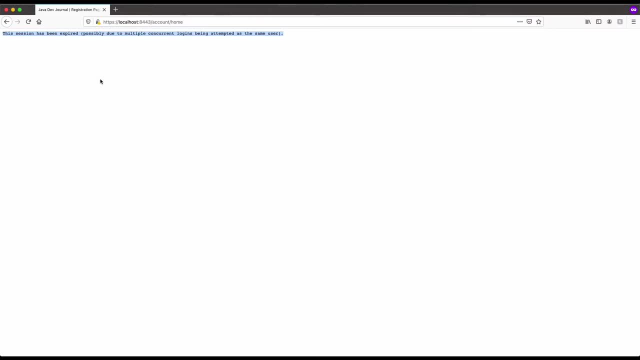 we're going to do this. let's go back to firefox and just see what happens if we set the maximum session- concurrent session- for the given user. what happened is spring security will allow you to log in from your second place, but it will invalidate your previous session, right? so the most. 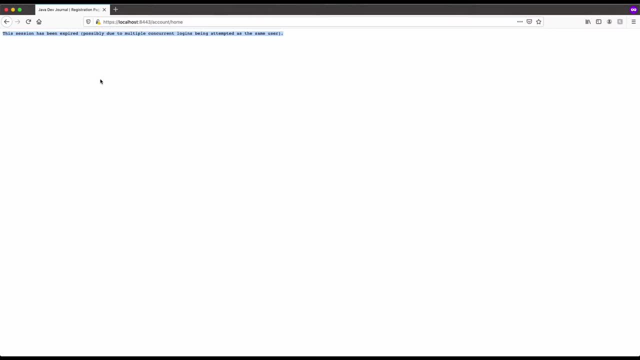 uh, recent login. uh attempt will be activated, will still be active from the spring security perspective, but your other sessions will be deactivated by spring security, but your other sessions will be deactivated by spring security. So there are two fundamental problems here. The first problem is: in many applications it's confusing. Think about it: You were working onto this Firefox doing some work, said accidentally, you logged in from the second browser or a different browser and then, when you take an action, you got this message, which is confusing As a user. I really don't know what happened, right? 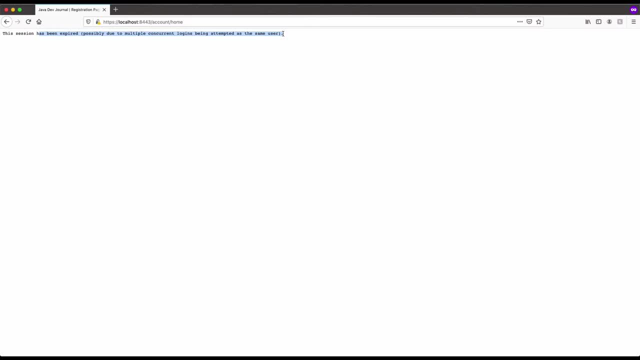 That's one problem. It's a problem. I will put it in a different way. It's not a very good user experience, But if you want to still continue that one, it's up to you. okay, Right? The second problem is: this is not something you want, right? 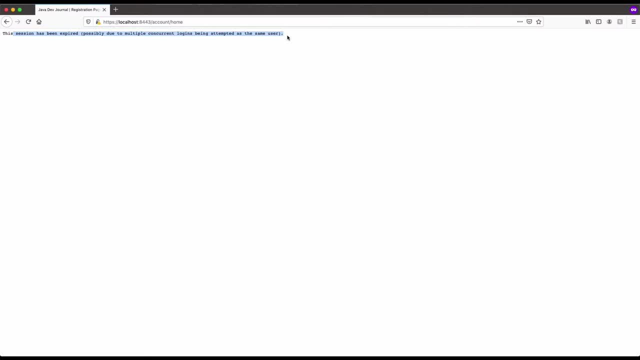 Your application might have a different look and feel and you want to adapt your error message. or you want to give a different error message and you want to redirect customer to a different screen. right, And that's a very fundamental requirement for any of the application. 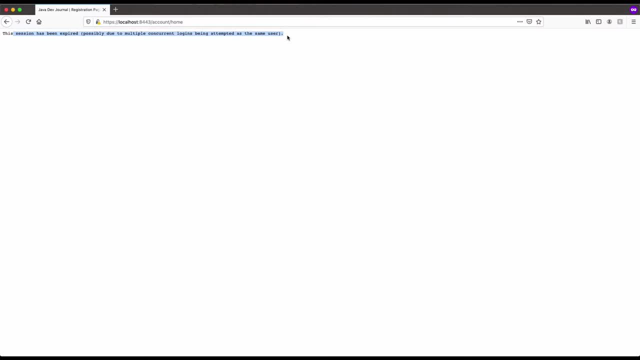 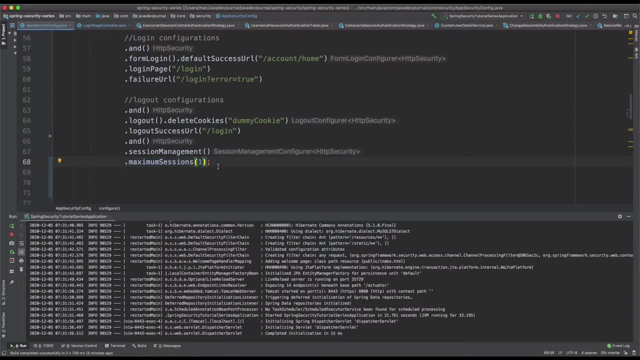 And for both the cases, Spring Security provides you the built-in mechanism where you can use the configuration same session management thing to control the behavior, right? So let's see what we can do for both the things, all right. So the first thing, what we are going to do is: 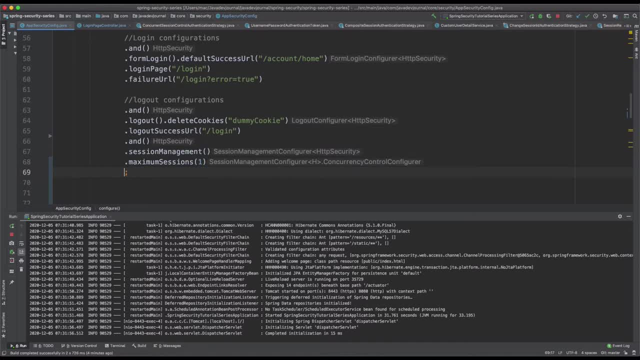 we are going to control that. what should happen if the maximum, if the customer, has already exceeded this configuration right? So for that one you can use the expired URL. This will tell Spring Security that, hey, when this happens, instead of showing that a default message. 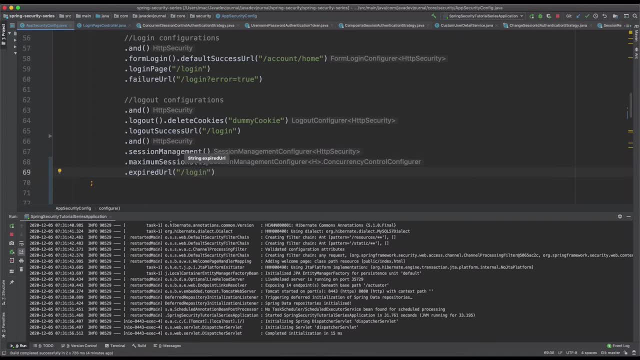 you should redirect customer to my login screen, right, And then you can always pass: invalid session is equal to true. This is the request parameter that can be passed. okay, So that's the first thing that you can do. So what is going to happen is when this case arises. 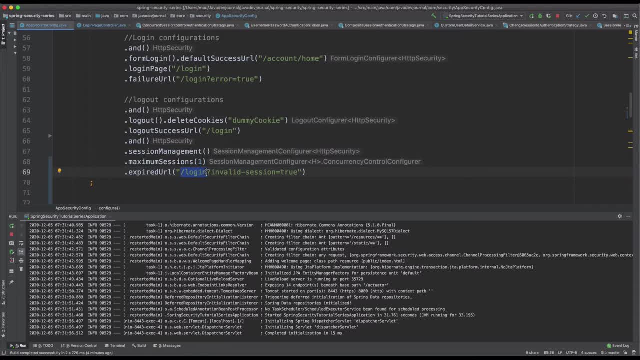 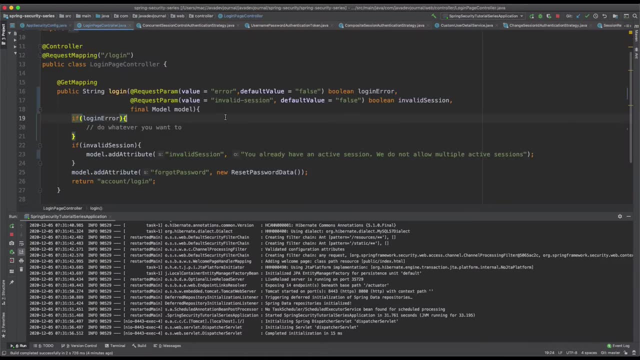 Spring Security will pass the control to login controller and will pass this parameter request parameter. right, If you look into our login controller, we are basically accepting this request parameter. It's an optional- and then if we have that one, I'm storing it into the model and returning to login page. 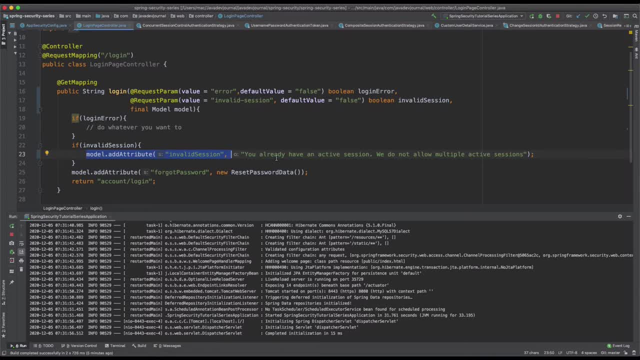 and in that login page I'm showing this message And so I have the full control. How do I want to show the message? If I want to show a different message, I can control that one, all right. So that's the first aspect of doing that one. 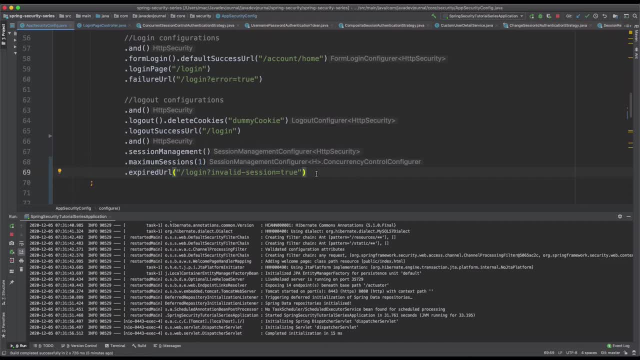 Now to get back to the second issue, right where what was happening is: my previous session got invalidated and the latest request was accepted, or the login request was accepted by Spring Security, right? So in order to handle that one, there is another configuration. 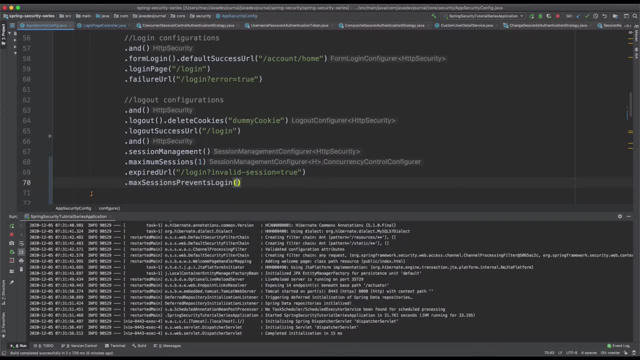 which says max session prevention, login is equal to true. okay, If this is active. if this thing is active, expired session URL will not work as per your expectation. So don't assume that if you are setting this session prevent login as true. 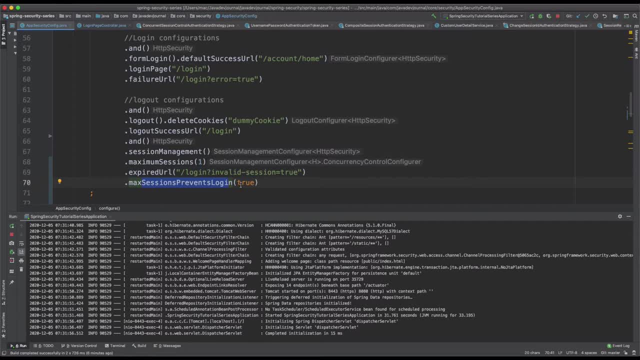 then again, with what we did earlier in our demonstration: customer will be redirected to the login page, And the redirection. the reason is: when you set this max session prevent login. So what has happened is you're telling Spring Security that for the second attempt, don't even allow customer to do a login. 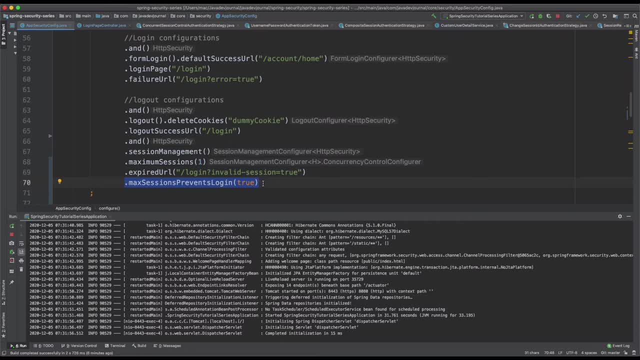 Instead of that, one show the login error message to the customer. So if I am logged into the Firefox and then I try to log in from the Chrome or a different browser, instead of having that behavior where I was able to log in from the Chrome, 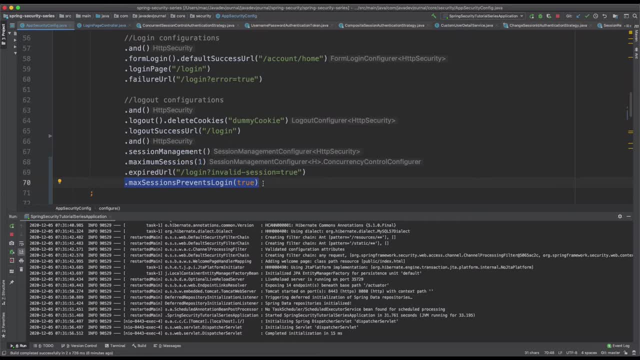 in this case you will get a login error message. So Spring Security will not allow you to log in from that Chrome browser. okay, So just to give you clarity that if this is set true, you won't be redirected to the invalid session thing. all right. 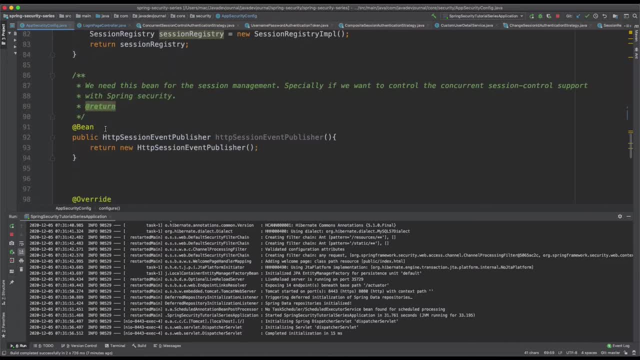 Another thing which we will be discussing in more details: in order for this entire functionality to work together and correctly, make sure that you have configured the HTTP Session Event Publisher. Now, this event publisher is an interesting thing, and Spring Security uses it internally. 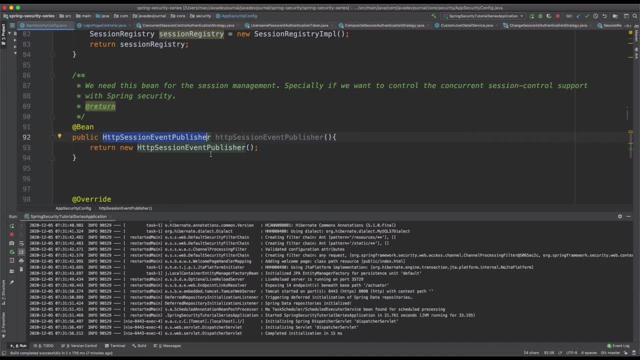 and we will going to talk about that one. So what happened is, with every session event, this publisher will publish the event and then Spring Security uses those events to take a call whether you should be allowed to log in or how many sessions we have, and all those things. 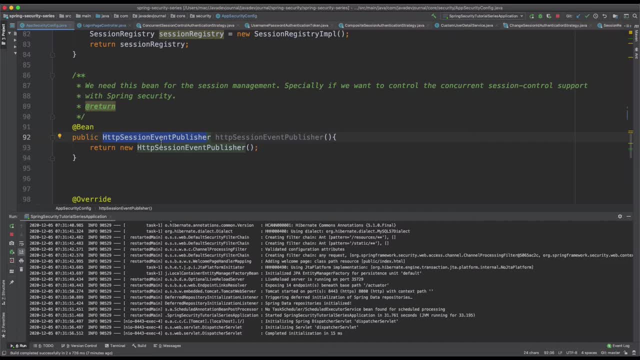 So, don't worry, I'm going to talk about that in this video itself. all right, Now, if you start your application and try to do the same exercise, what we did earlier- right, you will see a different behavior. So on your second browser you will get the login error message. 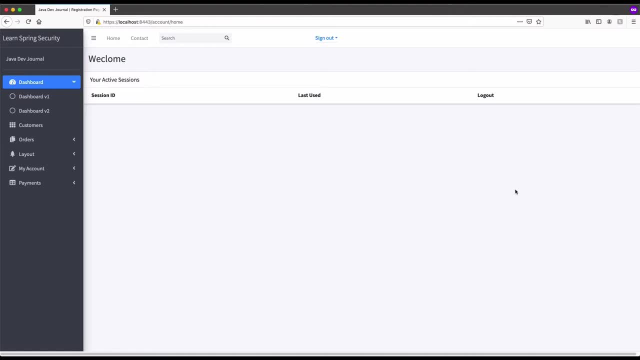 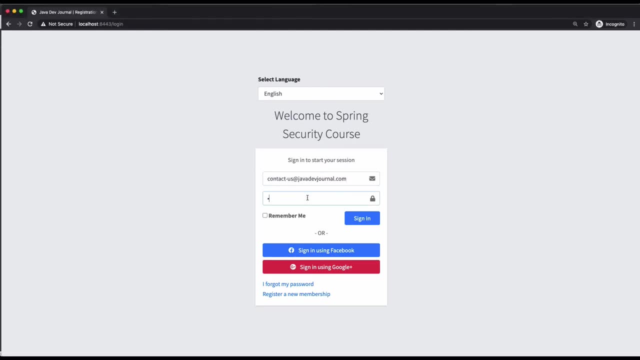 I restarted my application and now I am logged into the Firefox. right Now, let's try to do a login into our Chrome browser, okay, And if I try to do a login, you see I'm getting this username and password is incorrect. 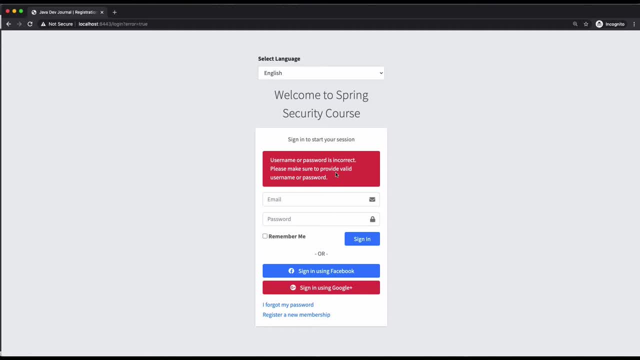 because I'm telling Spring Security that, hey, don't even allow the login from the second attempt, right? So continue with the current session and don't try to kind of invalidate my previous session and create a new session for us. 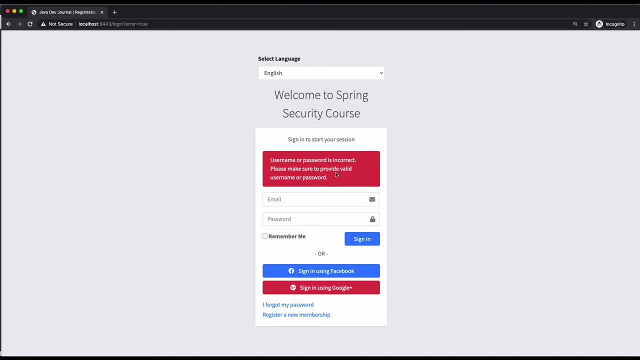 So that gives you an idea how you can control the concurrent sessions in Spring Security. There are different. There are different aspects. Just hold on that, and I'm going to talk about those ones. But now the next interesting question is how it internally works. 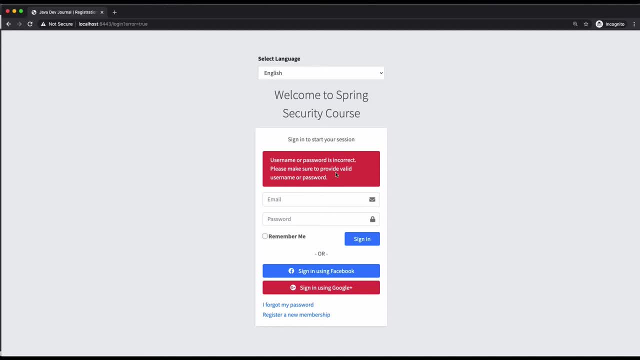 What are the different classes and what are the different filters and strategies? those are being managed by the. Those are being used by the Spring Security right. So, in order to understand, I am going to give you an overview, or the workflow. 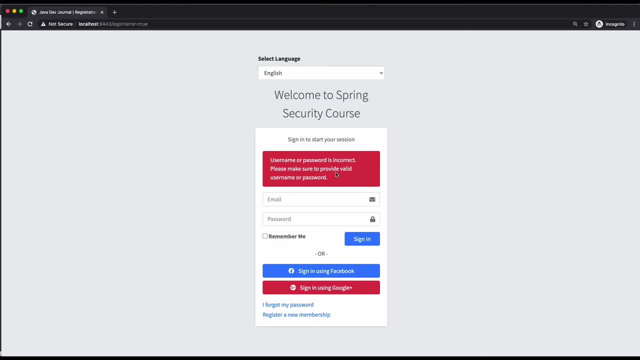 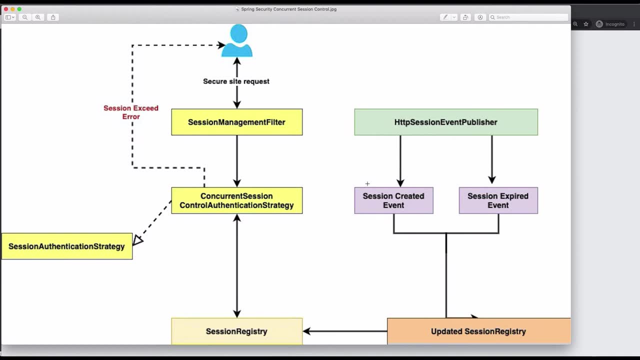 how it works internally, and I'm going to talk about the different aspects and then we will put out some debugger. So these are the points to understand it more clearly. So this is the high level of a workflow, how this entire functionality was working internally within the Spring Security right. 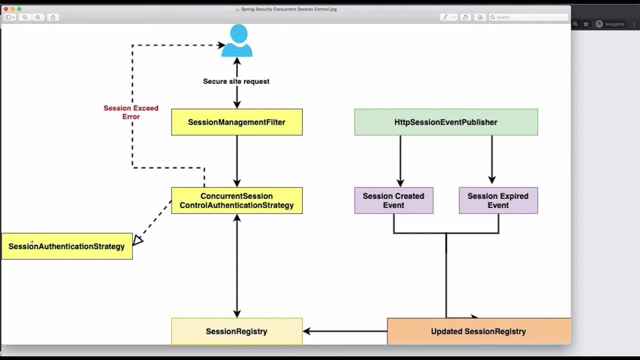 So we have a different. First of all, I'm going to talk about this section right, This one. So we have a different session authentication strategy. So this is an interface, right, And there are different implementations of this interface. all right. 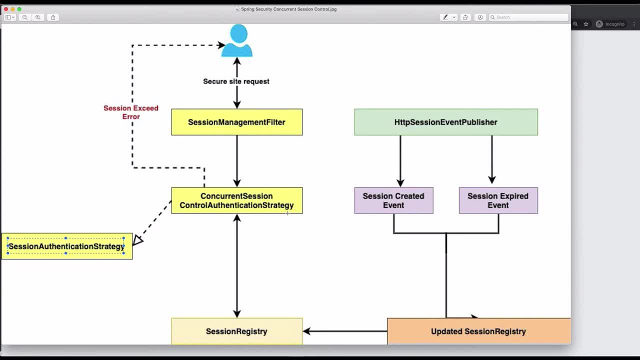 So session authentication strategy determines what should be my authentication strategy, So which strategy I should use when the user tries to log into my application, right? So that's the first thing. Session management filter is a filter which intercepts every request. 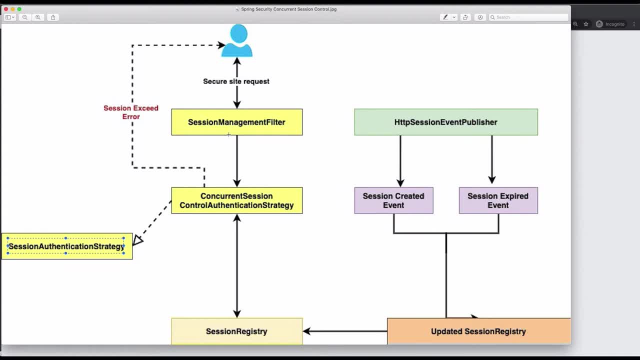 and then it basically handles the core mechanism or the authentication process to a session authentication strategy. Right, Because we are setting the concurrent control. So we are telling Spring Security that hey, use the concurrent session authentication strategy to authenticate the user. So concurrent session control authentication strategy will find out the different configuration. 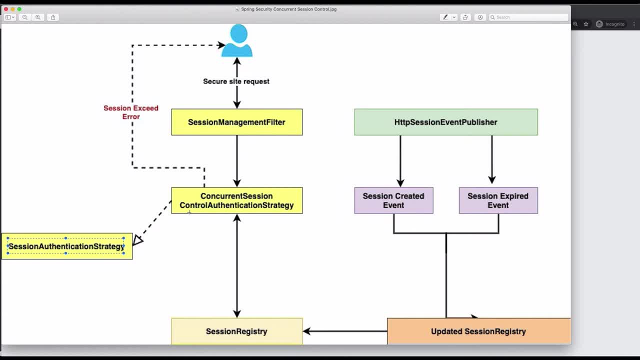 like how many number of different logins you are allowing for a given users, and then what are the different configurations- whether it should be onto the default or you have configured something different right Now. the other interesting thing is how Spring Security knows. 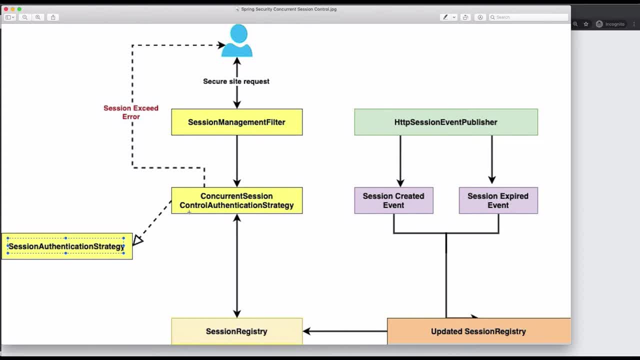 that, what are the different active sessions for a given customer and that's where the session registry will get into a picture. So the default implementation of the session strategy is: it's an in-memory. think of it as an in-memory map, Okay. 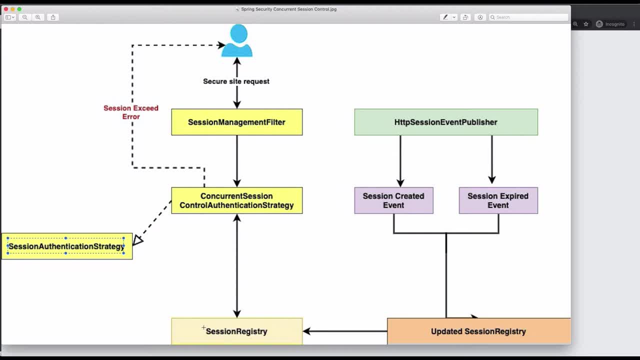 So this map contains two things. One is the session ID, and I'm just giving you a simplified view. It contains a lot of other different things, But on a simplified view, think of it as a map. It contains a session ID and then it also contains the information: who is the user? 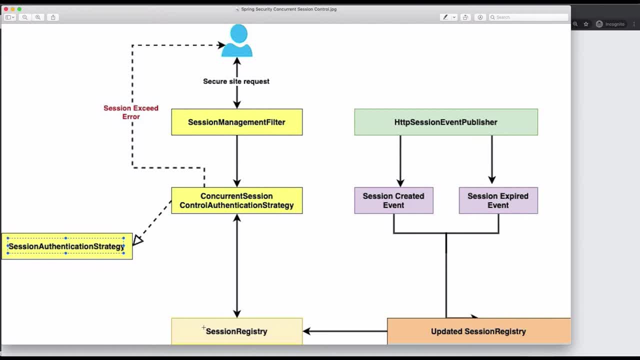 or who is the authenticated object with that session ID, and that authenticated object is nothing but a user information which includes your login ID. All right, So that session registry will- it will- keep a list of all the active sessions and who are the users associated with those active sessions, right? 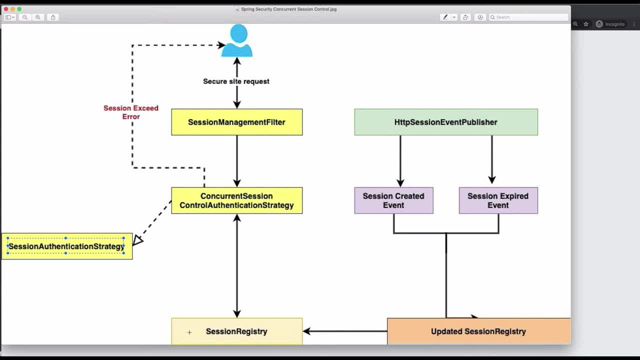 So now, if you are already logged in, there will be a record into the session registry which says user number one and here is the authenticated object for that one. Now, if you try to do a login from the different browser, correct. 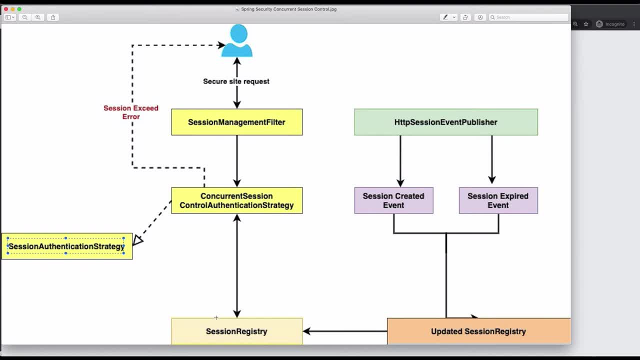 In that case, Spring Security will find out. hey, there is already an active session for you in the session registry. All right, So it will basically use this concurrent session control strategy, authentication strategy, and determine that, hey, this is not allowed. 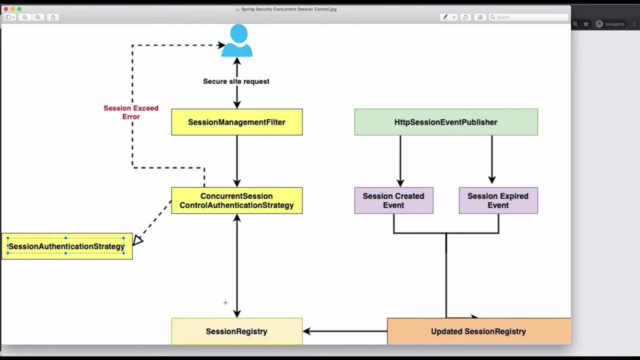 And now it will basically invalidate your request. All right, So in order for this session registry to be updated at the real time, that's where our HTTP session event publisher will get into picture For every session event, if a new session is created. 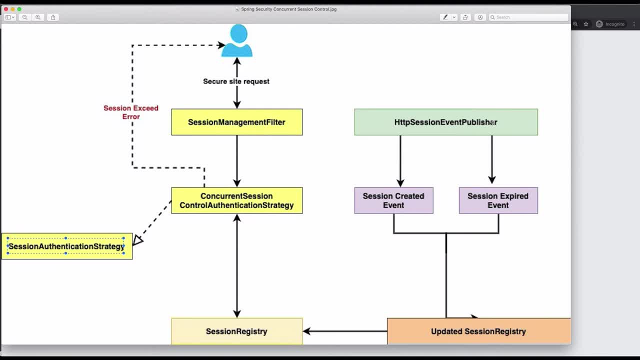 or if a session expired or a destroyed right. In that case, this event publisher will publish an event and that event will be updated into the session registry right. So if the login happened, you did a login for the first time. 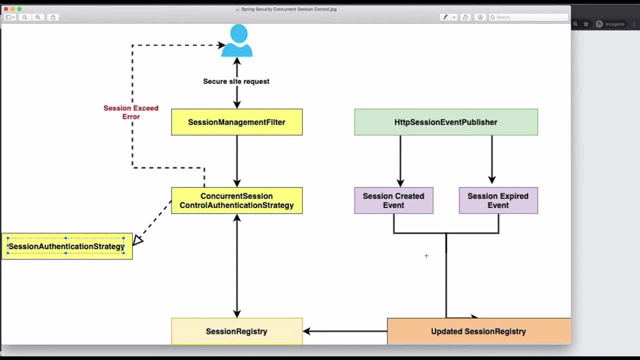 there will be an event, that event will be published and the session registry will be updated saying, okay, this is a session ID and this is the user. And if, let's say, you logged out or your session is in, 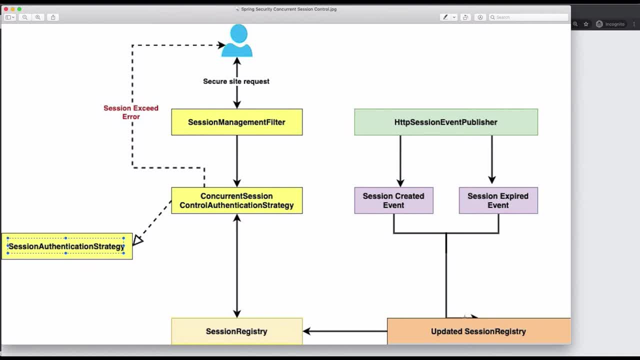 invalidated, another session event will be published and again, same thing will happen. So that gives you an idea. Now, to give you a more clear picture, what I'm going to do is I'm going to do some debugging around a one workflow. 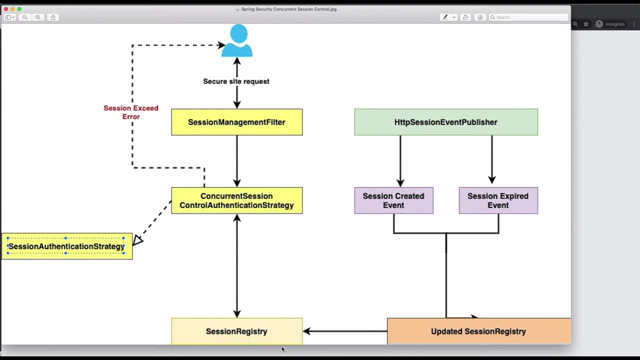 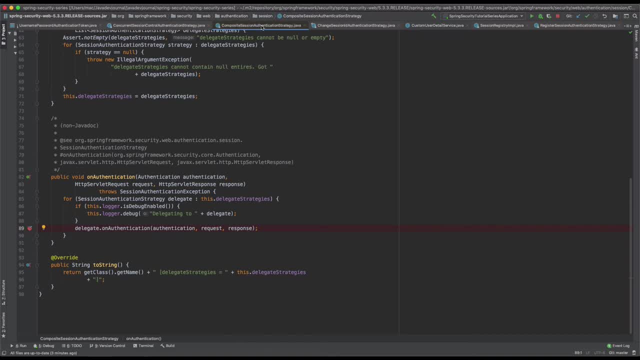 and then we'll see how it works. So, in order to understand, I have already put a few debugger points. One of them is onto the composite session authentication strategy, So it calls the different authentication strategies. In our case, it is going to call the concurrent session authentication strategies. 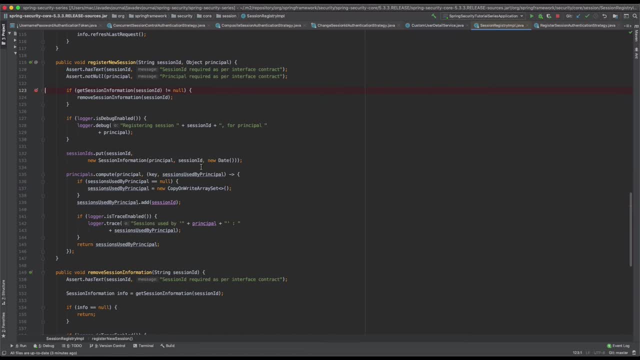 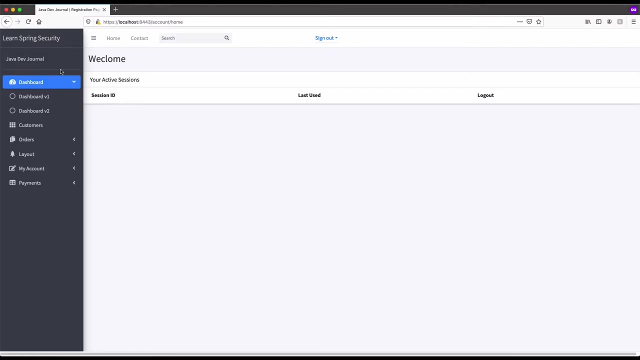 This one, right? I already have a session registry, right? This registry is basically keep track of all the active sessions and who is associated with that those sessions, right? So let's do one thing, okay. So, if you see, I'm already logged in from the Firefox. 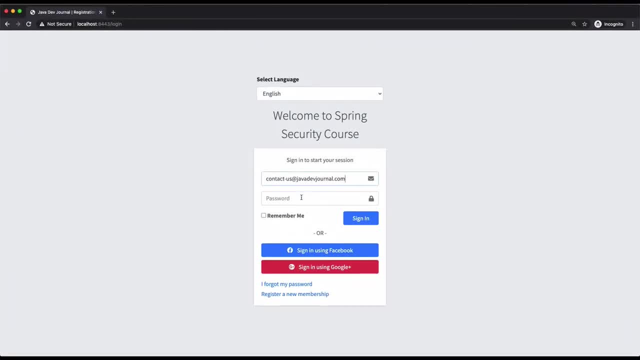 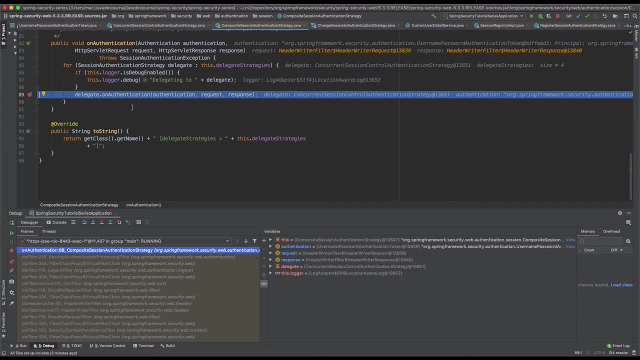 Now I'm going to log in from a different browser. okay, Let's do a sign-in. So I got into this method and, if you see, delegate is nothing but a concurrent session control authentication strategy. right, And that entirely. we dictate this one. 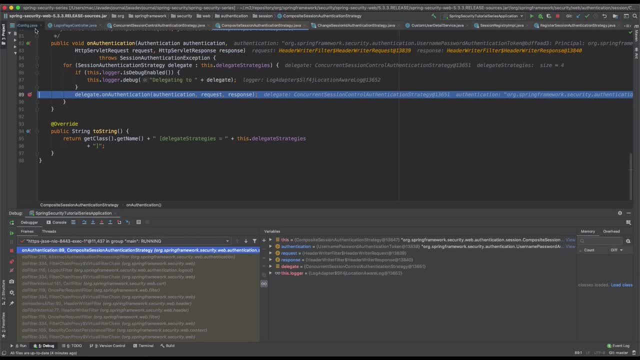 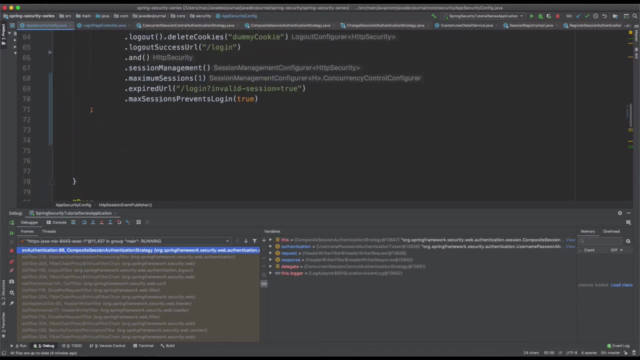 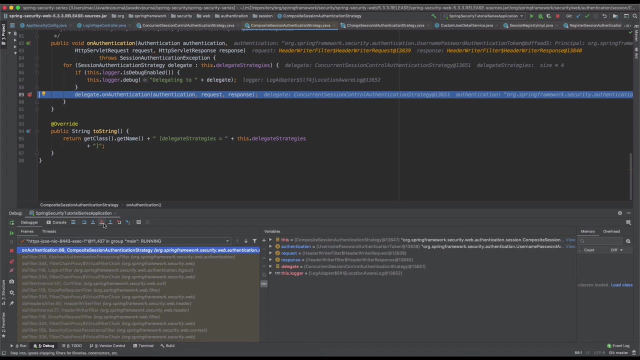 because we added that configuration. Let me close this one. We are telling the Spring Security that we use that session management thing and we use the concurrent session control thing. okay, So let's go back to our- And I'm going to get into the method, okay. 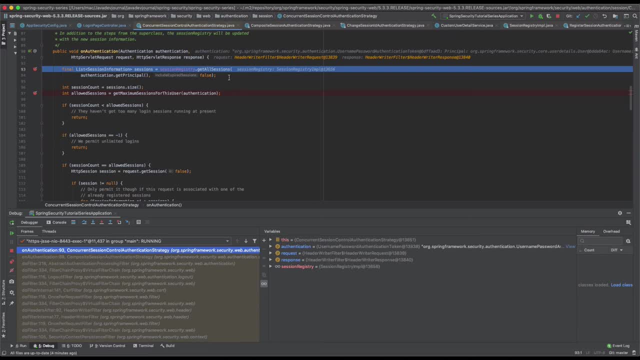 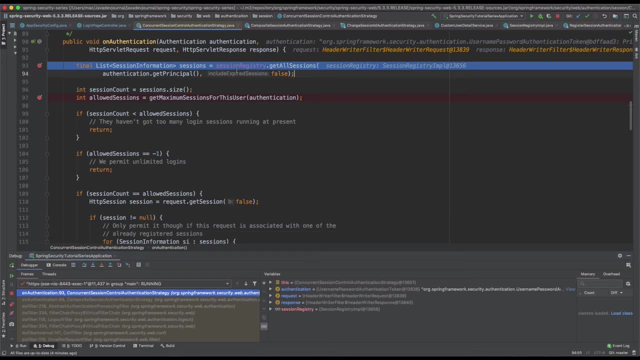 Now in my concurrent session control authentication strategy, let me increase the size a little bit. okay, The first thing, what I'm going to do is, if you see it is for authentication principle, it is going to see how many sessions are there for this given principle. 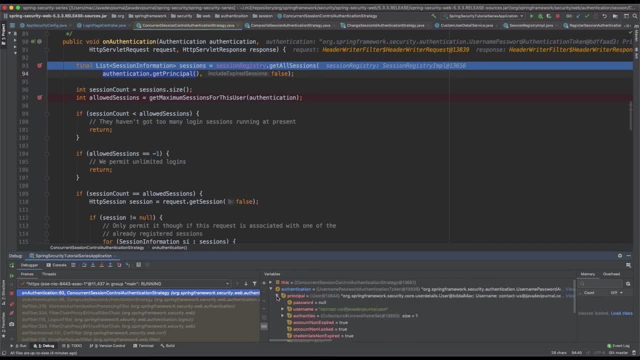 and this principle is nothing but the information which we are passing on. right, And this is contact us, the same login ID, right, You can go to this session registry, but what is going to happen is, in this case, it will say: I already have one session. okay, 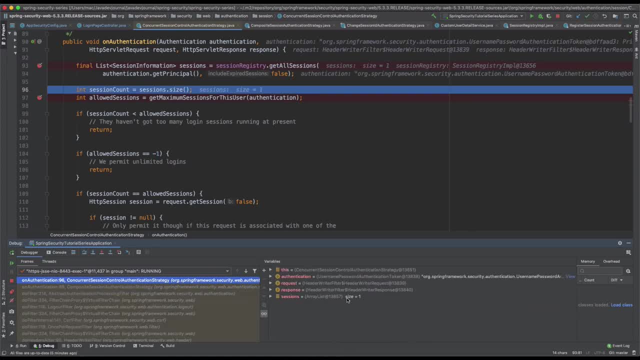 Let's close this one and you see, session is one, because I'm already logged in from the Firefox and you can get into this detail, this method: session registry. This is nothing but a session registry. IMPL. right Now it says that I have a count as one. 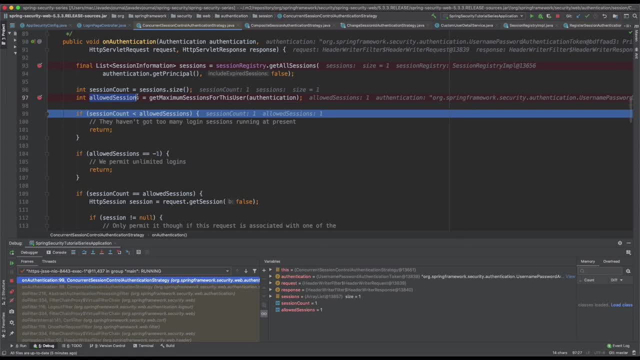 and then what are the allowed count? And again, this is we are dictating in our application, so we are allowing maximum session as one, so session is not less than so. this condition will be false. minus one is the default configuration. 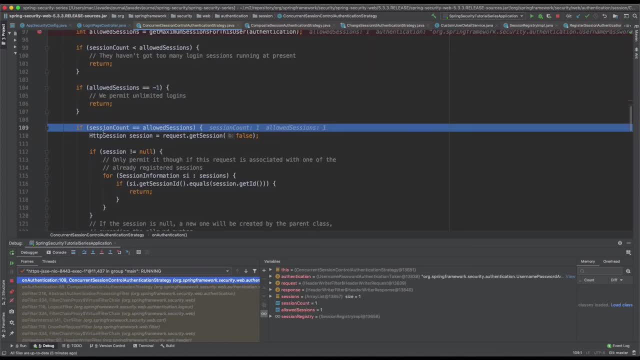 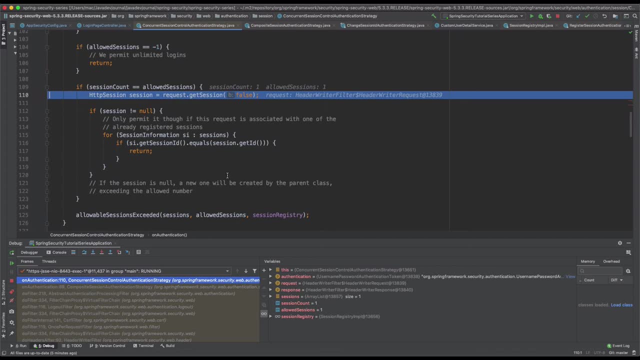 If you don't specify it, this will be false. and now this is where we fall. right Now we are into a situation where it says that we have X kind of a get into position where we have already exceeded the allowed configuration. 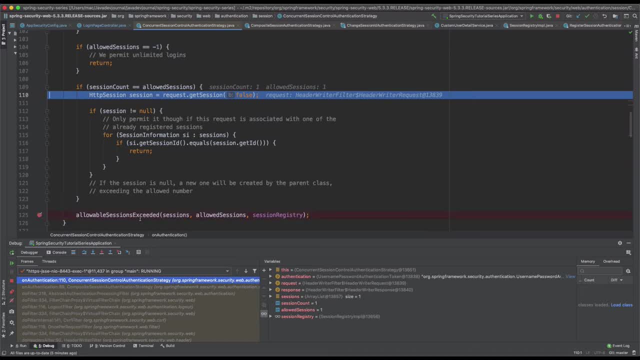 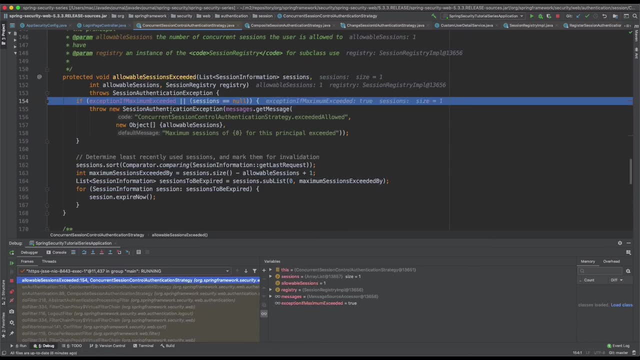 and in that one the control will go to allowable session exceed strategy. And if you go inside this one, there are a number of different things. to save some time, I'm not going to talk about it. You can always look into concurrent session control strategy. 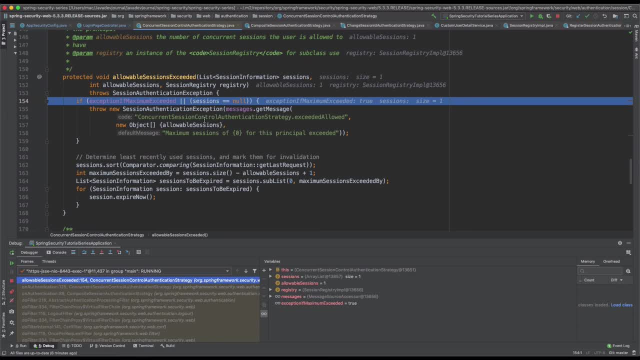 but what happened? is it basically find out all the sessions, sort it out and then it takes a call which session it needs to invalidate, right in case of a default behavior, and should it allow or should it not allow. so you can go into those details. 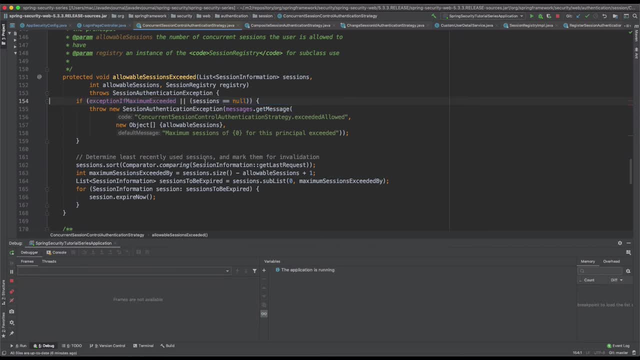 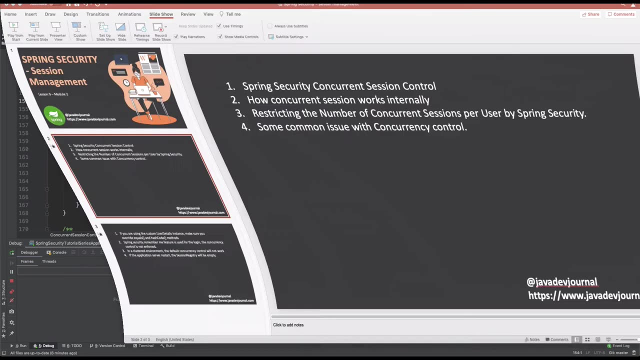 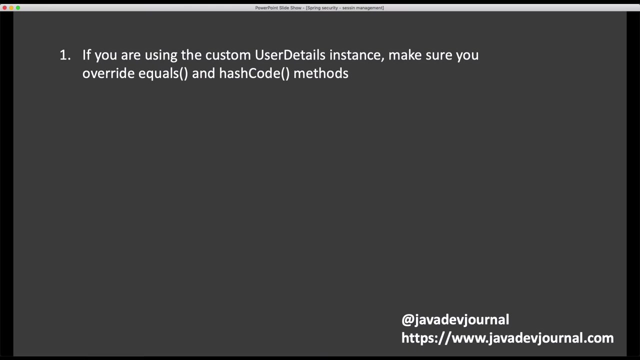 but the idea was to give you an understanding that how internally it works. right, And at the end of this lesson, I'm definitely going to talk about a few other things. okay, If you're using it, there are a few things which you should be very clear. 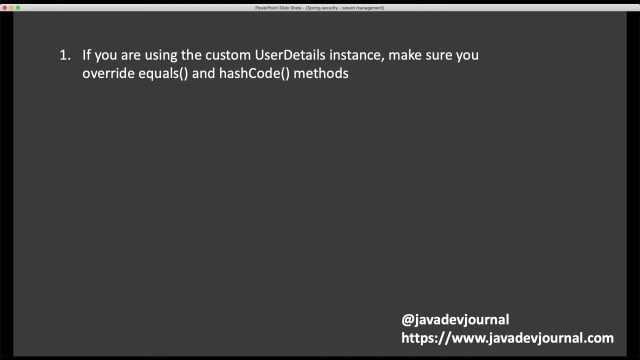 For example, if you are using a custom user detail object and for most of the enterprise application, you will end up creating your custom user detail object. This is object where Spring if you're using a custom user detail service. if you have not, you don't understand it. 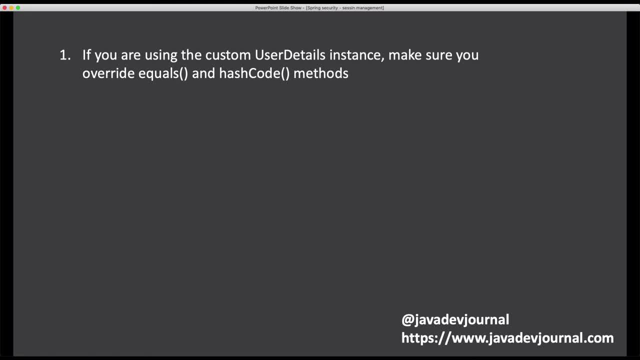 go back to my previous lessons. This basically give. this is an authenticated object which is written by Spring Security. So if you have created your custom user detail object, make sure you overwrite the equals and hash code method And the reason for that. 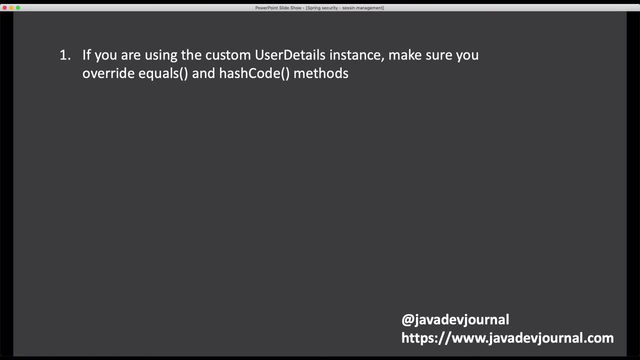 that one is, if you remember, I was talking about the session right Where Spring Security tracks all the active session, the session registry. it's an in-memory map And in order for it to identify the authenticated user, it needs the equals method to identify that one. 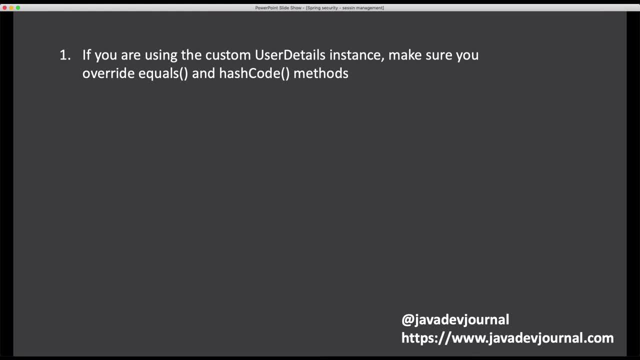 And any wrong implementation or no implementation will give you a wrong result, So it will not able to identify those details. So make sure you overwrites equals and hash code methods right. This is, this is a fundamental requirement, okay. The second thing is, which is sometimes confusing: 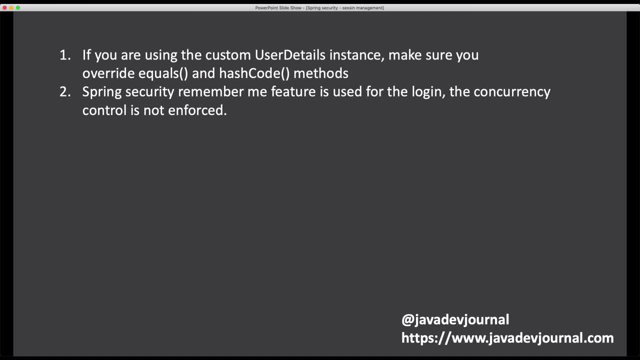 If you are using the default implementation right, The remember me functionality will not be part of the this session control thing. So if you are logged in from a one browser, let's say it's a Chrome, right On on your Firefox. 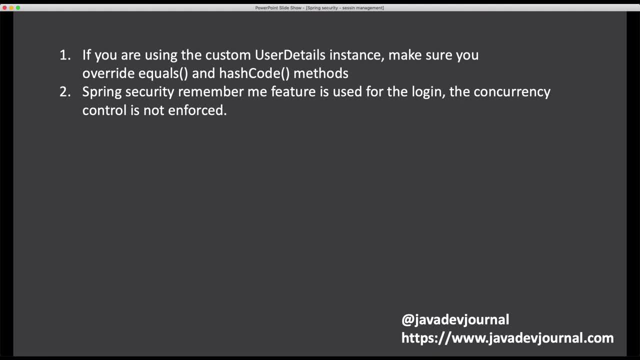 when you did your last login, you use the remember me functionality right. So now, if you're already logged into from Chrome and you open the Firefox, it will auto login using the remember me functionality. correct For this one: the default configurations. 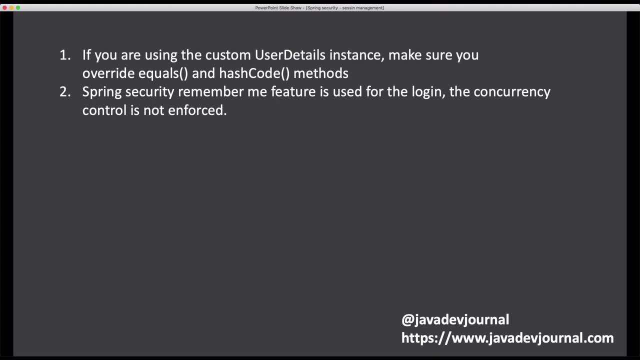 the setup will not work. That means your concurrent session control will not be enforced and the user will be logged in from the second browser. That's a. that's one of the fundamental issues. So you should be aware of that one. And there are some. 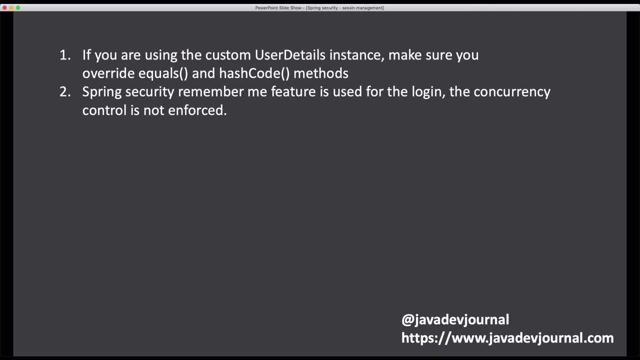 some techniques to handle it. I'm I'm going to talk about those ones, right. The other thing is the clustered environment. So if you are onto the clustered environment, the the, the default implementation again will not going to work, because 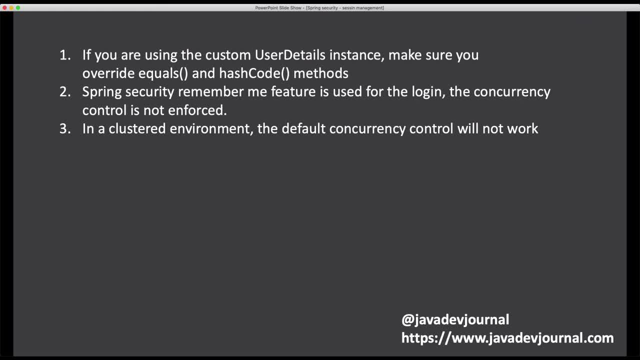 uh, session registry, as I said, right, So it's an in-memory implementation. So every cluster will have their own registry and the the maybe the different cluster will not have information about their in-memory map, right? So that's another problem. 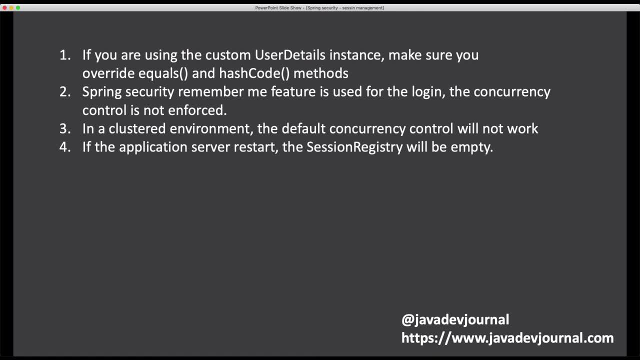 Uh, the other. there's an another problem. if your application restarts, right, So that means your session registry will be empty, So it will be. all the data from that session registry will be gone because it's an in-memory right. 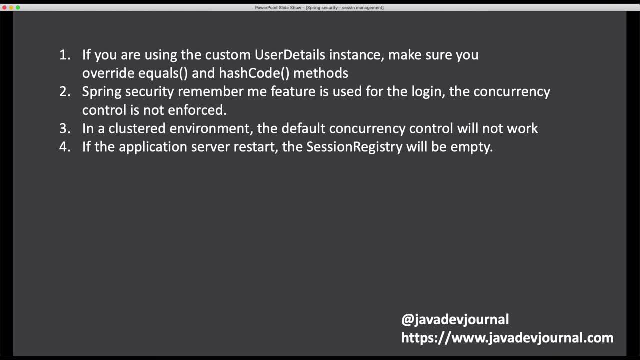 Uh, and then what happened is because the sessions are controlled by the application, uh server, right, So it start and you refresh the browser, You will be auto logged in based upon that J session ID, right? Uh, that's how the entire application works, but from the spring security sessions. 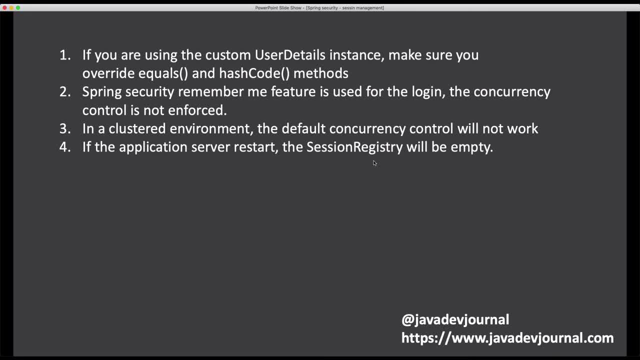 history perspective, it will still be zero, So it will. basically, there is a memory leak or there is a disconnect, right? Uh, so you will be logged in, automatically logged in, but session is yesterday. We'll say it's zero.